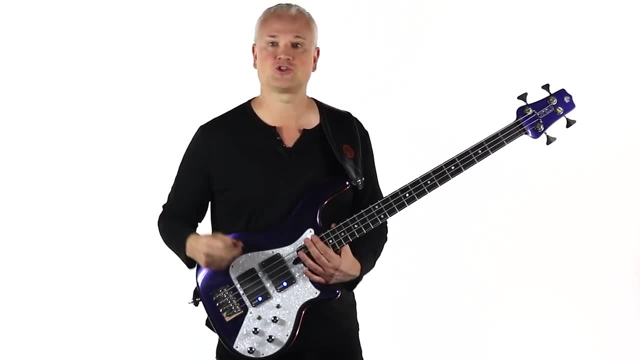 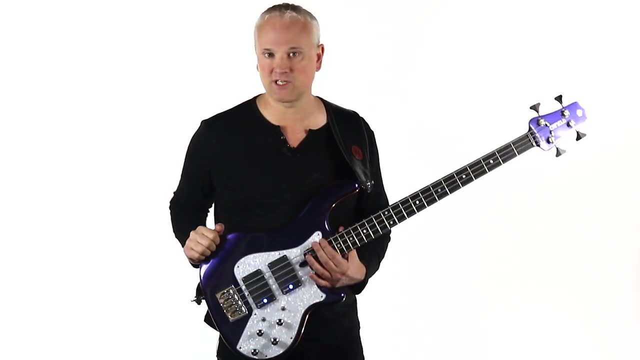 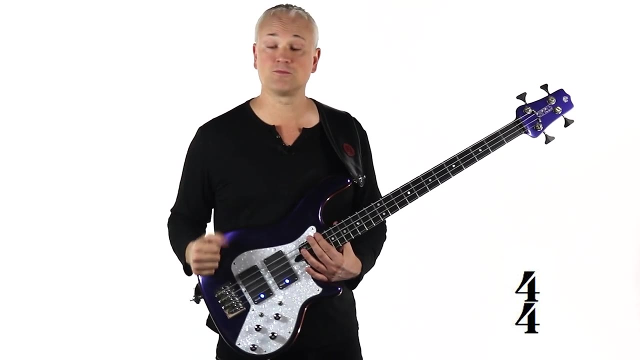 Each cycle is called a bar, So one, two, three, four is a bar, And the number of beats in each bar is signified by the time signature. A time signature has two numbers. The top number, which is the numerator, is the number of beats in a bar. The bottom number, the denominator, is the type. 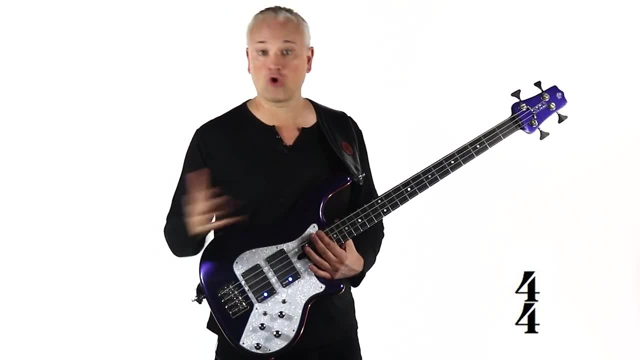 of beat, So that could be quarter notes, half notes, eighth notes, all of which we'll look at in a second. But the key to understanding time signatures is to think of them like a fraction: Four, five, six, seven, eight, nine, 10,, 11,, 12,, 13,, 14,, 15,, 16,, 17,, 18,, 19,, 20.. 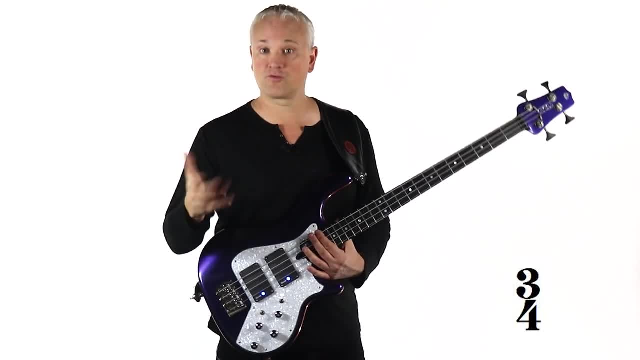 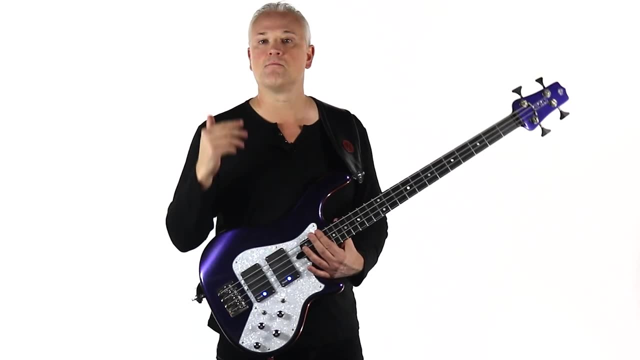 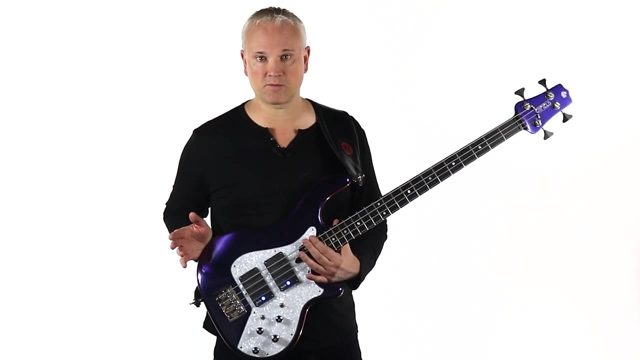 Four. four is actually four quarters Three. four is three quarters Four. two would be four halves Six. eight is six eighths. But like I said, we'll look at those rhythms in a second. If we want to count some bars of music out, we also need to know the tempo or speed of the piece. 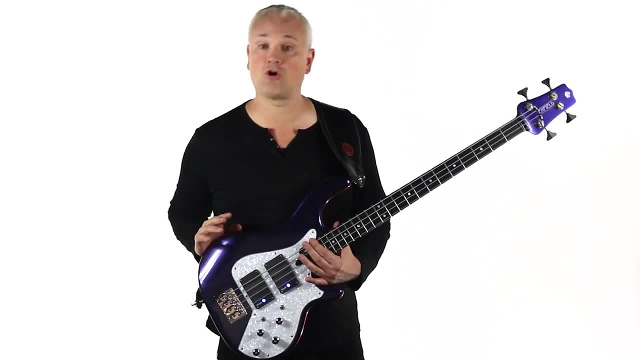 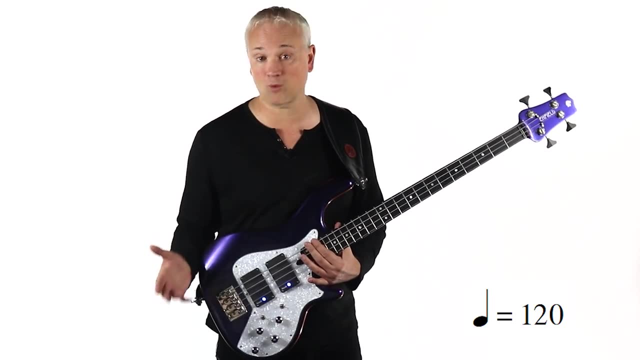 You might see Italian terms such as adagio or allegro or andante, But in more modern music you're more likely to see a metronome marking like quarter note equals 120. So for 120 beats per minute, we're going to have a pulse that's going to be somewhere around. 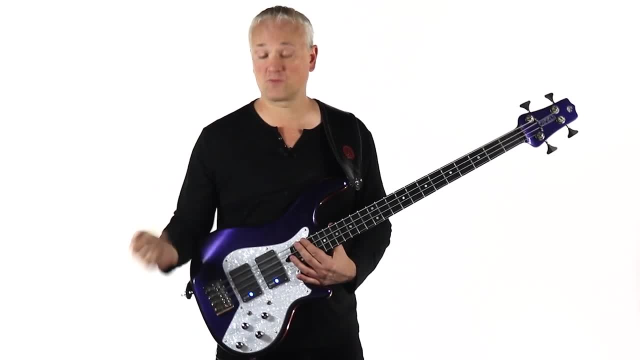 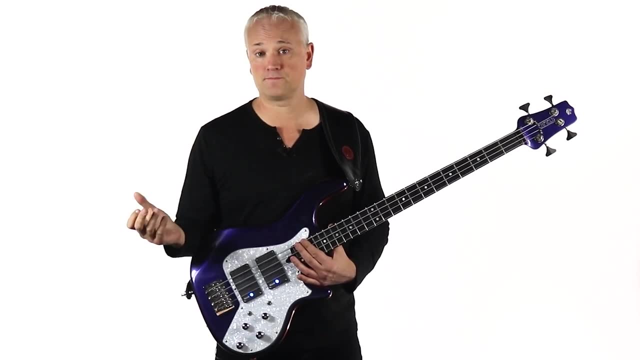 one, two, three, four. one, two, three, four, And then 60 beats per minute would be half that. So one, two, three, four. A faster tempo like 220 beats per minute would be a quick pulse like. 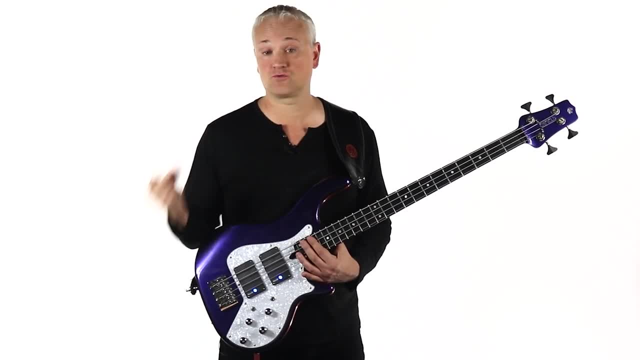 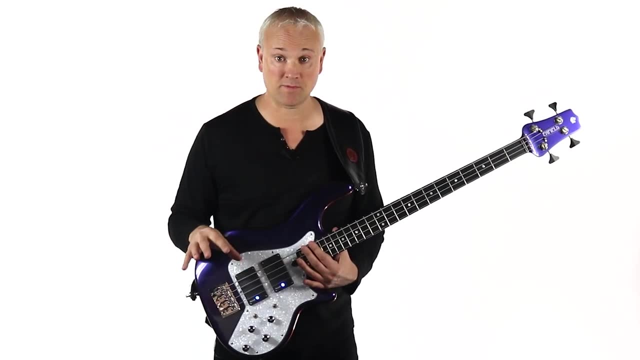 this: One two, three, four. one two, three, four. one two, three, four. So that's the basic background to musical rhythm, But that's only the general pulse. That's how we count bars. We haven't added any individual notes into the mix yet. Next we need to look at some rhythms. 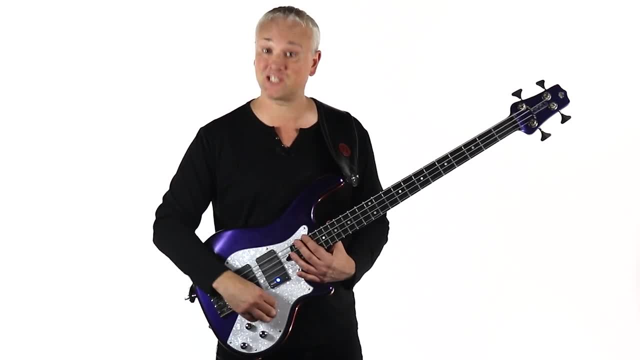 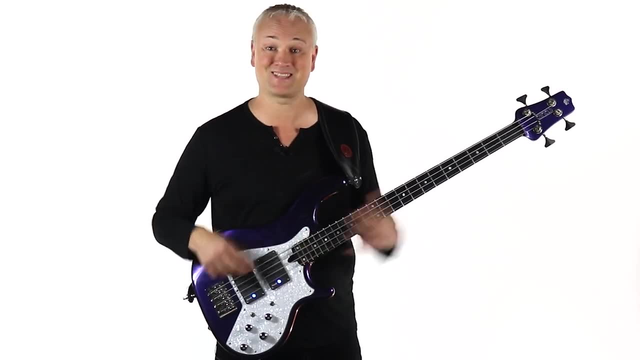 Now I'm going to introduce each rhythm in turn and use a single note of C at the third fret of the A string. for demonstration, We'll work through a succession of rhythmic drills where you can just play that single C note using the rhythms provided. That way we're looking at the 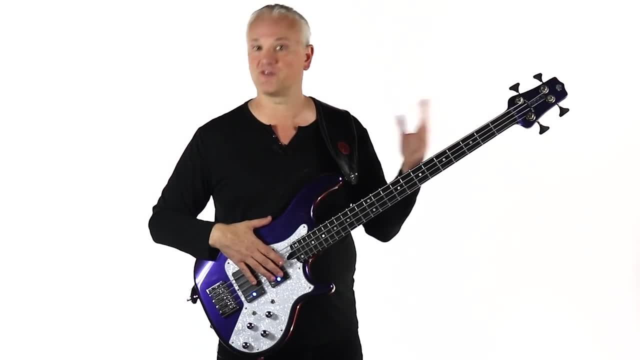 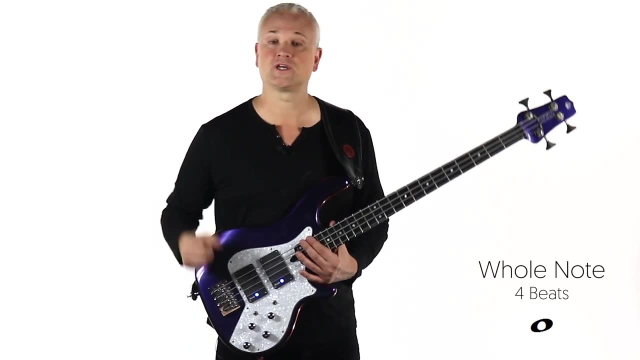 rhythm in isolation. All of these drills will be in 4-4 for ease of understanding and at a slow to medium tempo. First things first. we have the most basic of rhythms, The whole note. Now. this is four beats in length, so it lasts a whole bar of 4-4.. 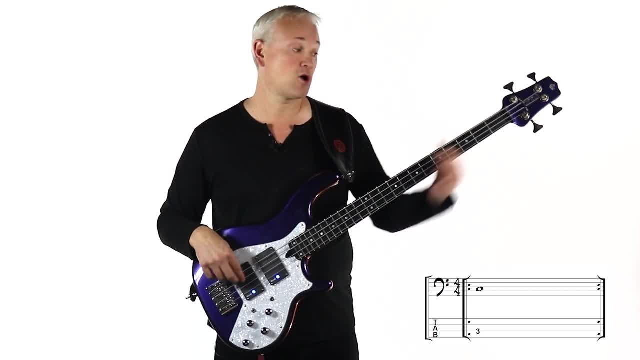 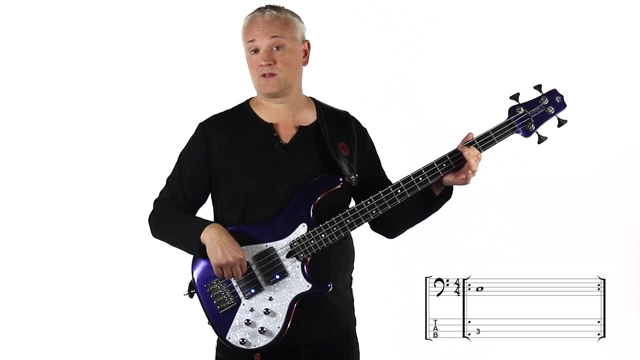 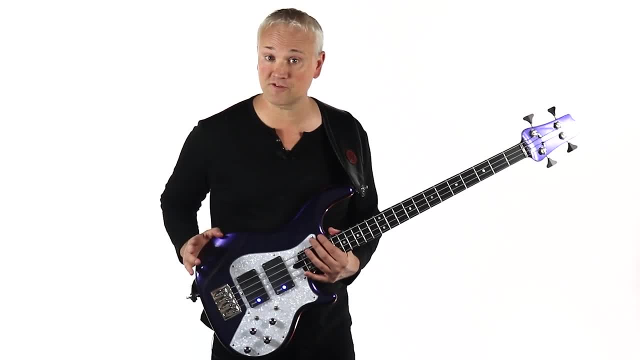 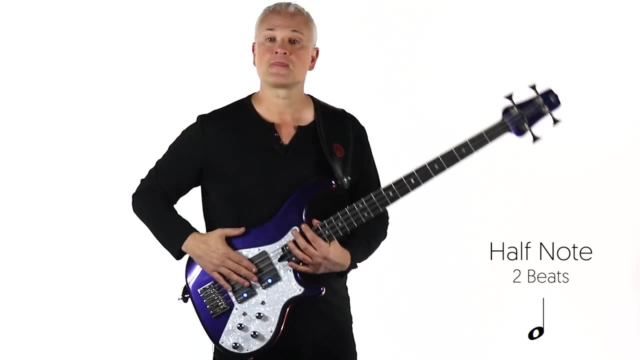 and then we just count out four beats. Next up we have the half note. This is two beats in length, so it's half the length of the whole note, obviously, And it's an empty oval shape with the stem. For one half note, we're going to count 1, 2.. Simple, so just two. 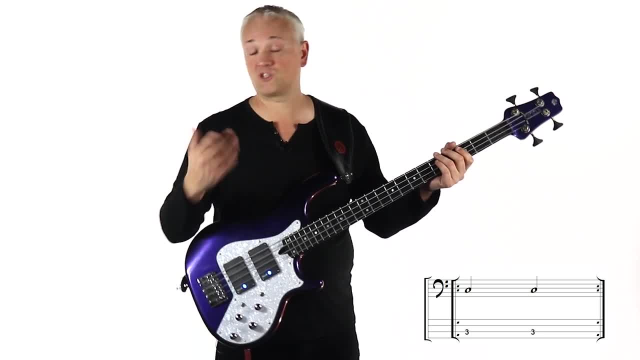 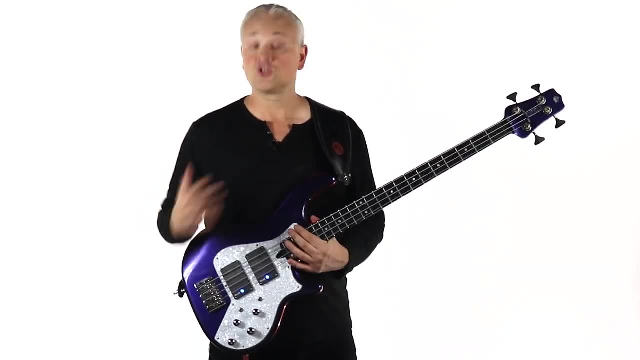 beats And we can play two half notes in one bar of 4, 4,, which would be counted like this: 1, 2, 3, 4, 1, 2, 3, 4.. So now we have whole notes and half notes. 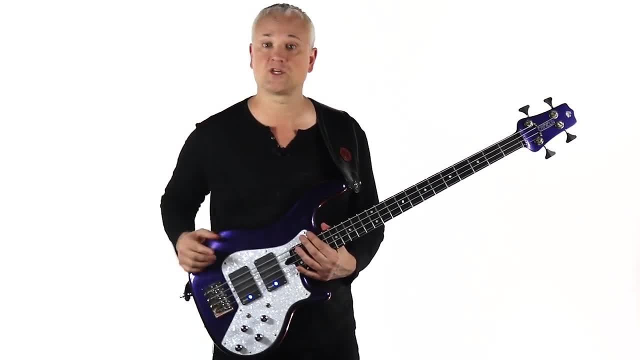 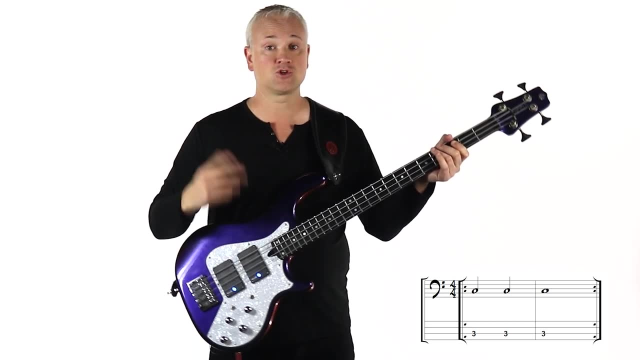 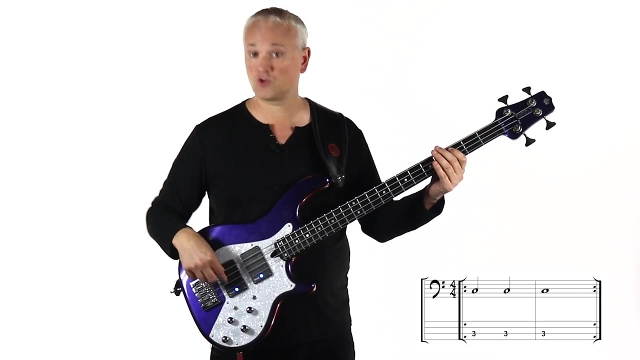 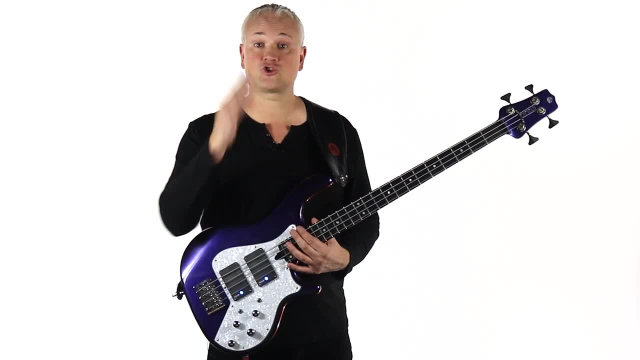 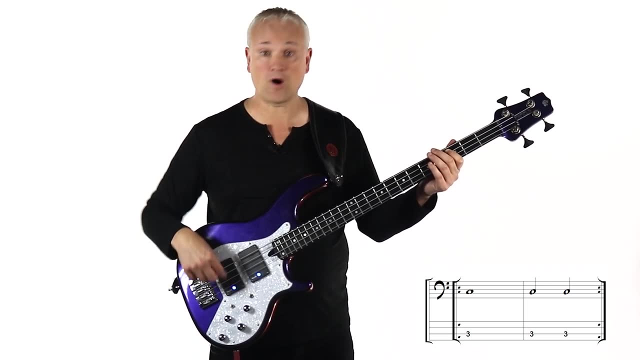 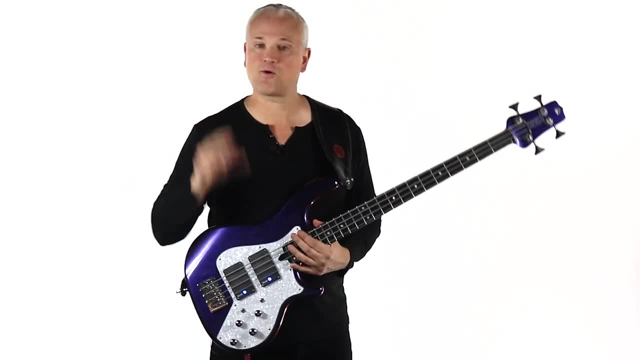 1,, 2,, 3, 4.. Easy, Notice how I'm not using a metronome or a count. I'm just using a metronome. So I'm just using a metronome, So I'm just. 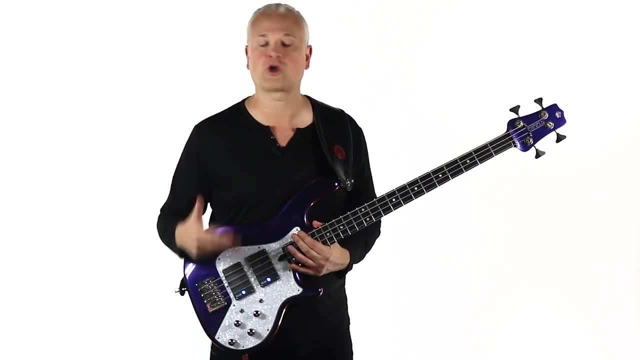 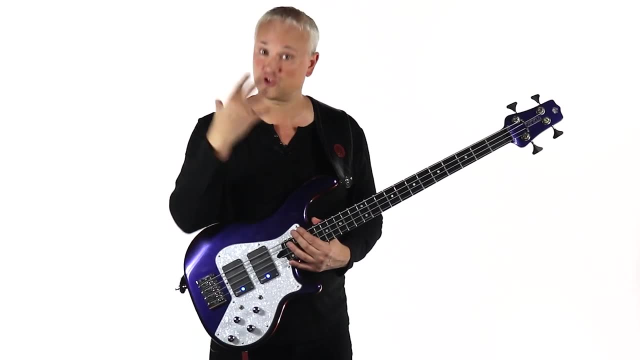 using a click for this. It's just to develop your own counting internal clock. You don't want to feel any pressure from outside sources. This is just about looking at those rhythms, understanding what they are and just learning how to count them. 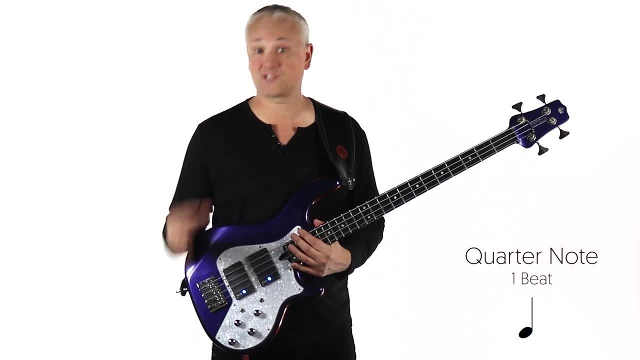 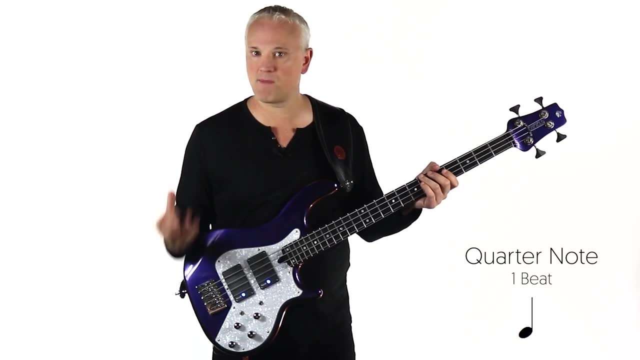 Next up, we have the quarter note and this is the basis for our 4-4 time signature. Remember what I said about the time signatures: It's like a fraction, four quarters. So this is four quarter notes And this is our main pulse. This rhythm is. 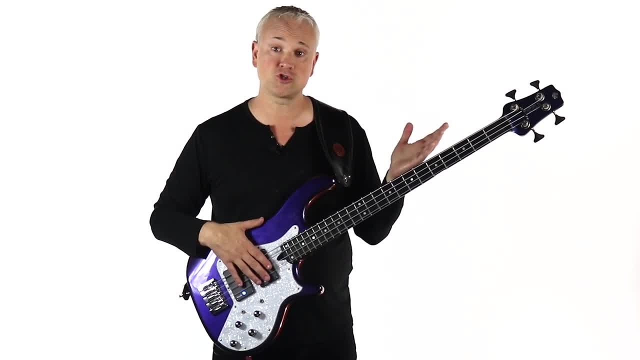 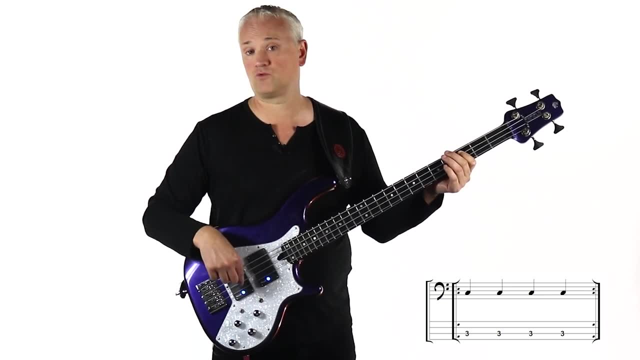 written as a filled oval with a stem. So with four quarter notes in a bar, we simply play it on each beat like this: 1, 2, 3, 4, 1, 2, 3, 4.. And obviously, if it was at, 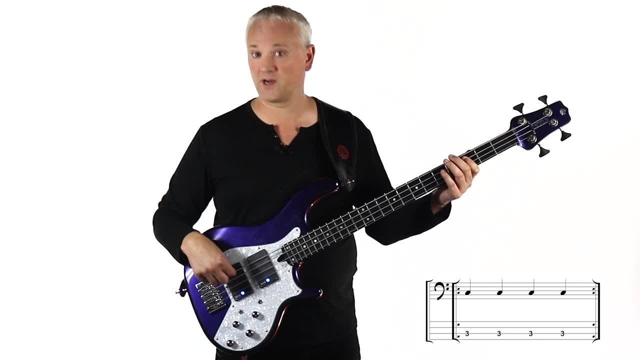 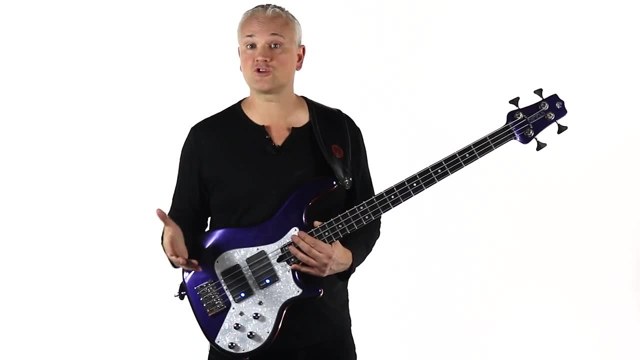 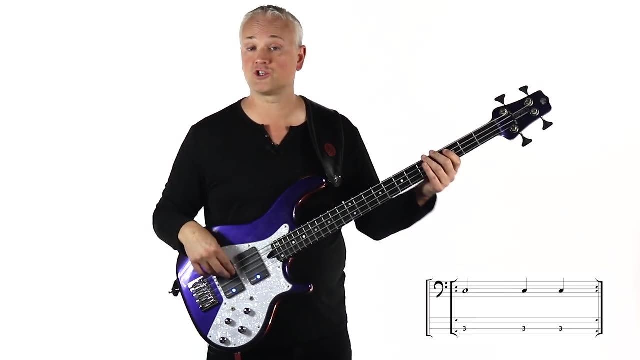 a slower tempo: 1,, 2,, 3,, 4.. Obviously, all of this is based on relative to the tempo. So now we have a half note and a quarter note. we can try combining them with these next two drills. So first of all let's just take a half note and then two quarter notes, which? 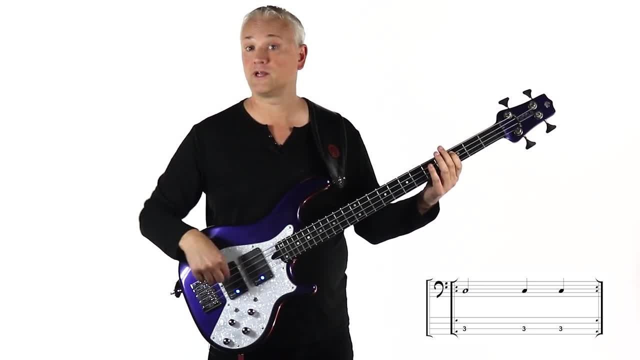 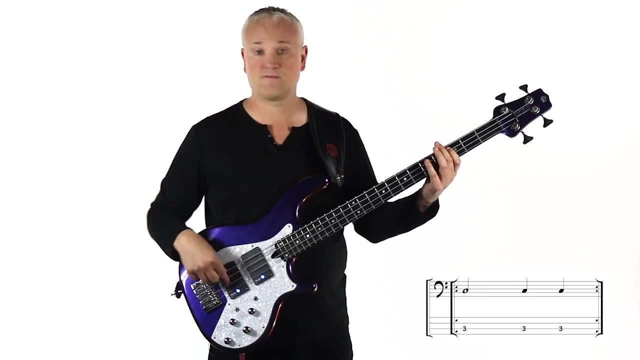 is going to be counted like this: 1, 2, 3, 4.. So if we go round and round, 1, 2, 3, 4, 1,, 2, 3, 4, 1, 2,, 3,, 4.. And then we can try two. 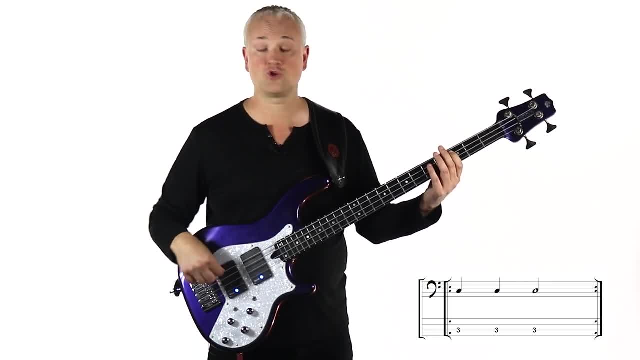 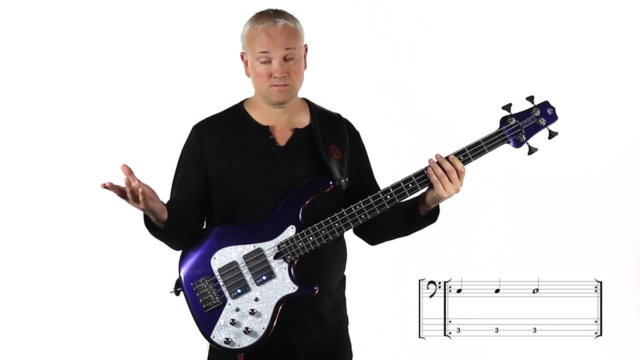 quarter notes and a half note, which you count like this: 1, 2, 3, 4, 1, 2, 3, 4, 1, 2, 3, 4.. Simple, You'll notice that for each rhythm we've halved the length of the. 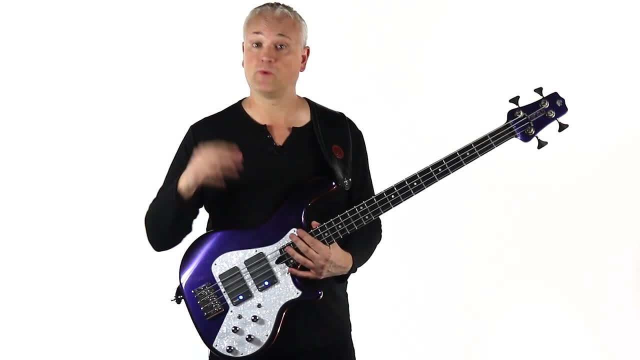 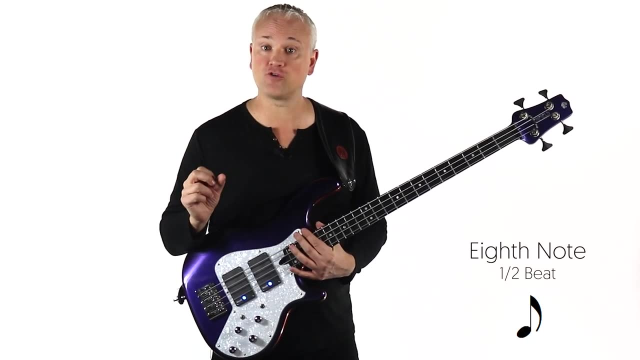 previous one. So we halved the whole note to get a half note. We halved the half note to get a quarter note, And if we halve the quarter note we get an eighth note And this is shown as a filled oval with a stem and a flag. So one eighth note has a. 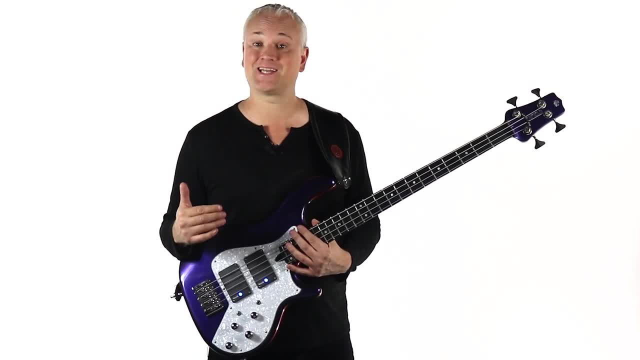 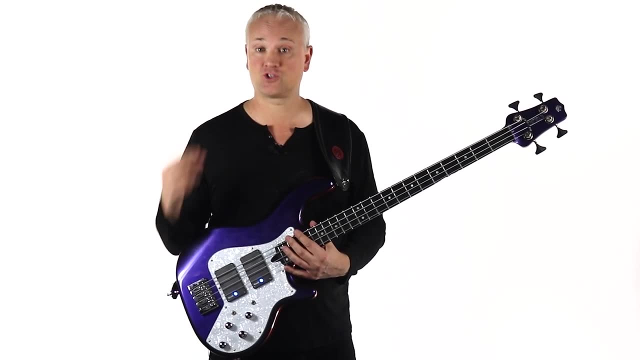 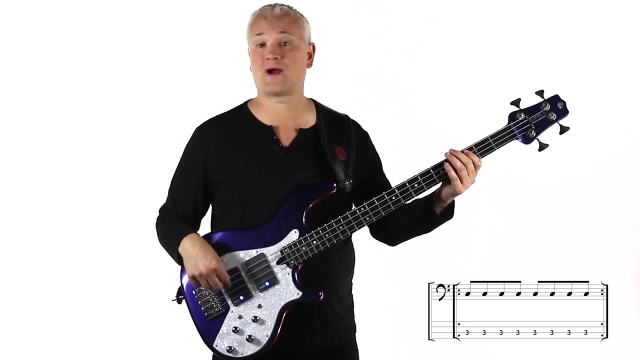 flag written like this, and then two or more eighth notes are connected with a beam. So we basically straighten up that flag and we count eighth notes as 1 and 2 and 3 and 4 and So, playing them while tapping the foot on each beat, 1 and 2 and 3 and 4 and So. 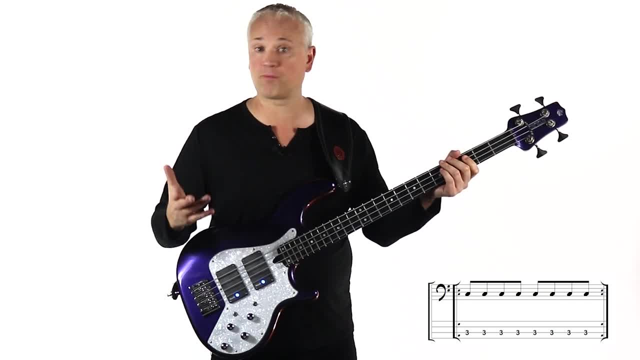 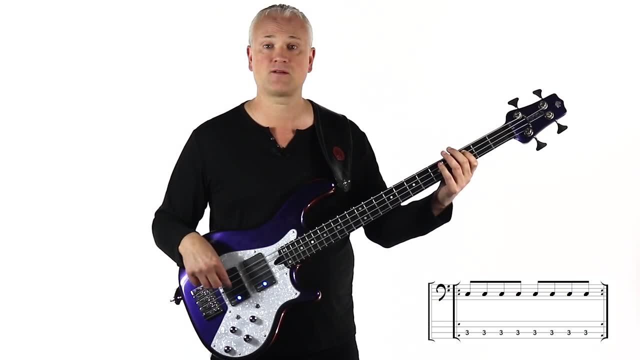 we're adding a count in between each beat. So again for a full bar of 4-4,: 1 and 2 and 3 and 4 and 1 and 2 and 3 and 4, and- And it's important to keep counting with your foot. 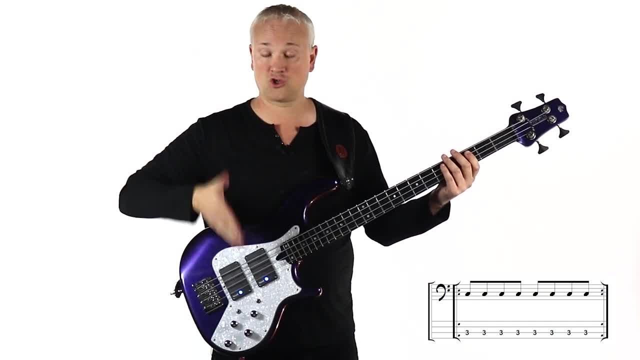 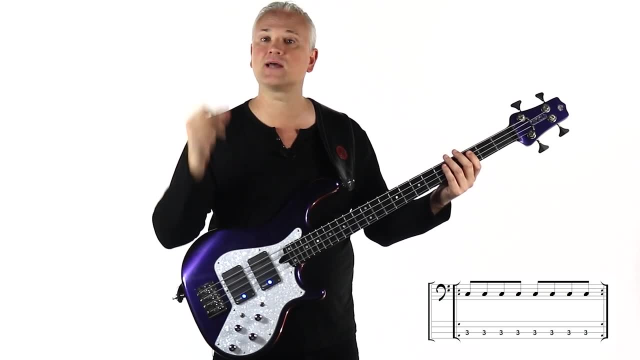 on each beat. So the foot is on 1,, 2,, 3, 4 while you're playing 1 and 2 and 3 and 4, and That click there takes the place of the foot or the head. nod, or whatever you want to do. 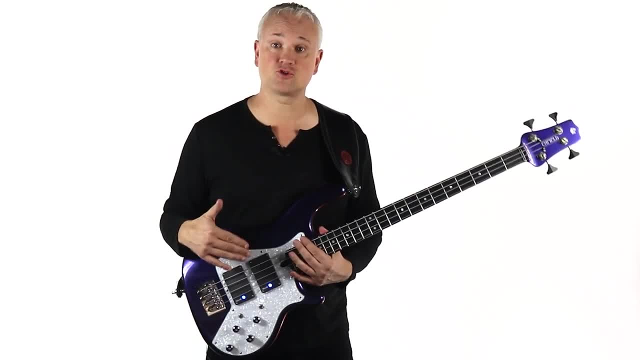 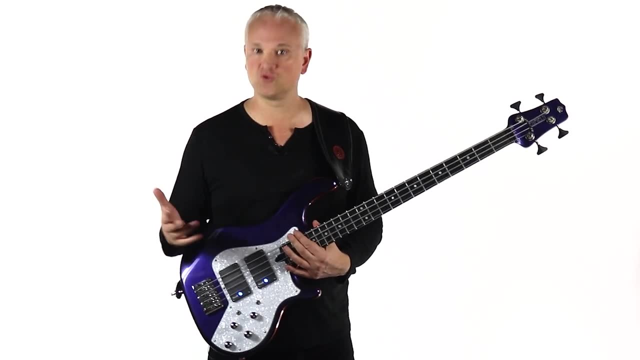 1 and 2 and 3 and 4, and, And just as we combine the previous rhythms, we can now add the eighth notes into the mix with our quarter notes and our half notes. So let's try some drills using various eighth note rhythmic cells. So for the first one, let's try quarter note. 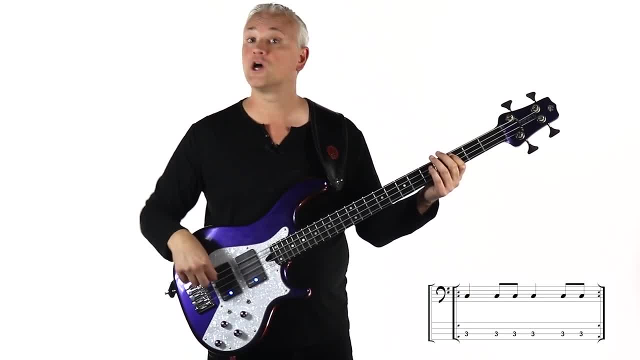 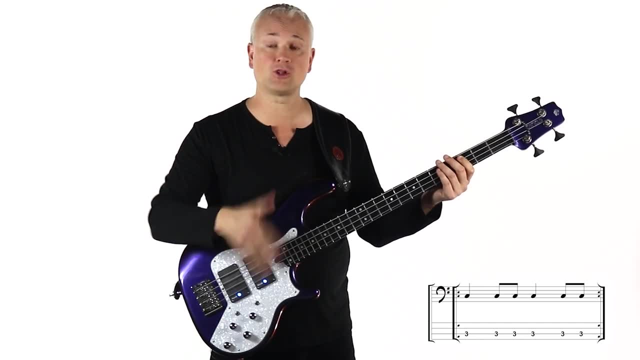 and then two eighth notes. So we're going to count that as 1, 2, and So for the full bar, 1, 2 and 3, 4, and So you just read them along as you get to each beat And you can. 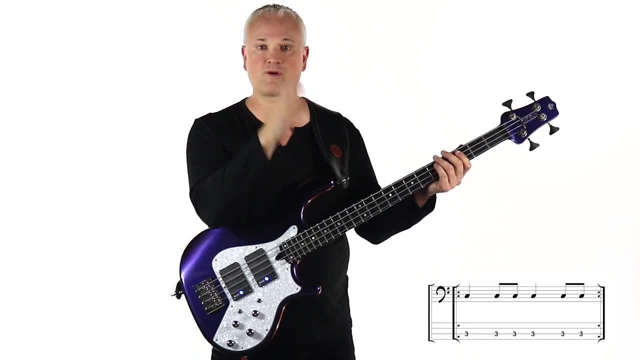 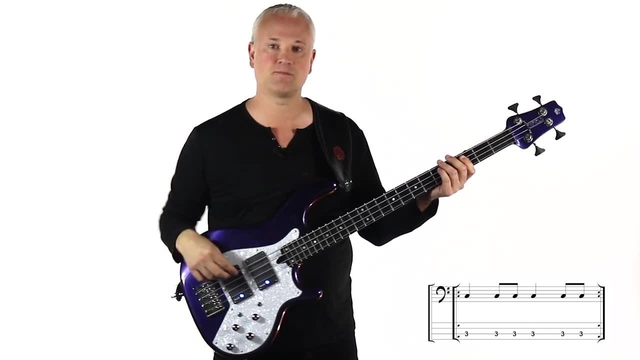 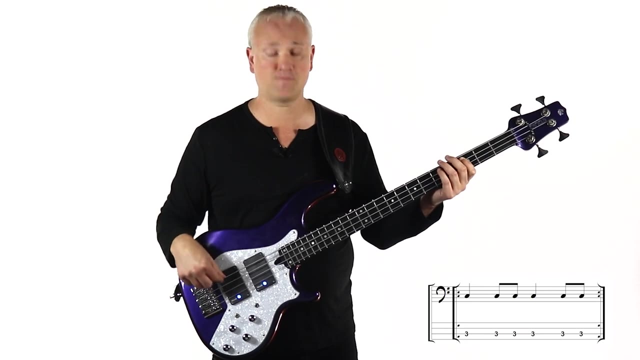 see how It comes in the music. It's all very segmented by beats. You can see the outlines of the beats as you work through the bar. The eighth notes are there connected by the beam, So 1, 2 and 3, 4, and 1, 2 and 3, 4. and Now let's try two eighth notes and a quarter note. So 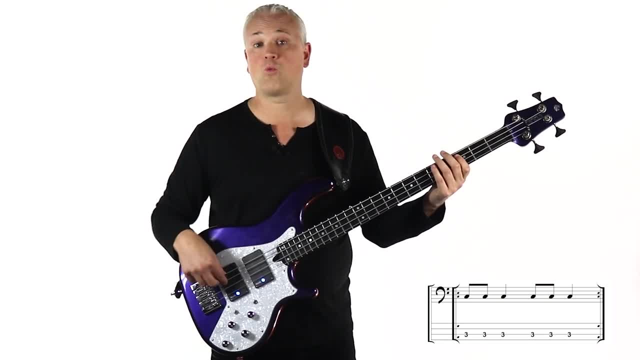 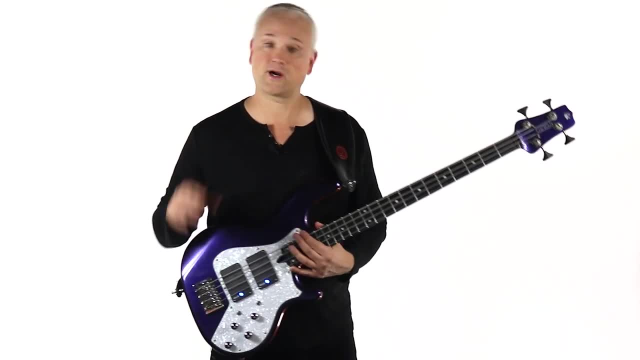 that's going to be 1 and 2.. And then for the full bar: 1 and 2,, 3 and 4, 1 and 2,, 3 and 4.. 1 and 2,, 3 and 4.. 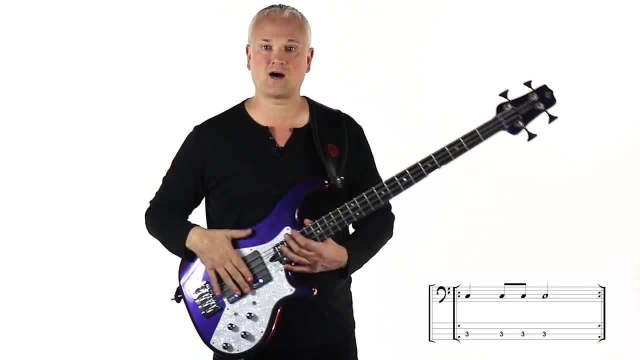 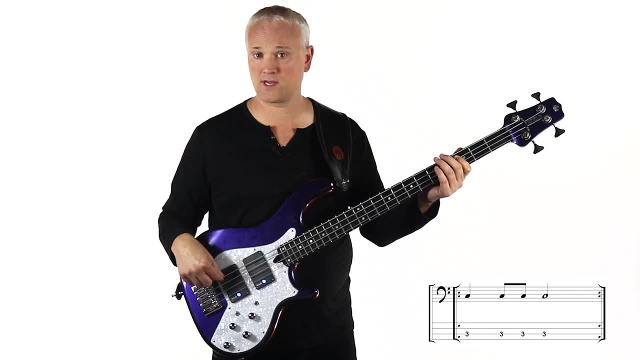 And then there's a half note in there. So first of all, let's try quarter note, two eighth notes and a half note, which we're going to play as 1, 2 and 3, 4.. 1, 2 and 3, 4.. 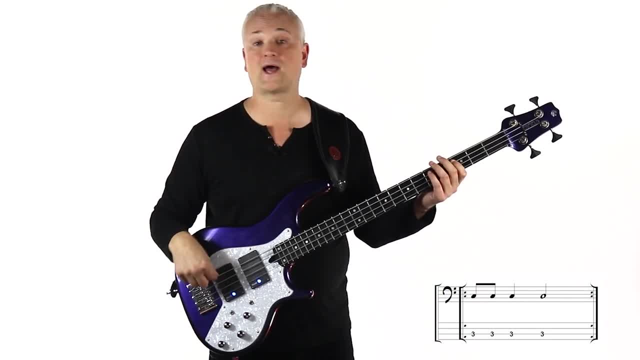 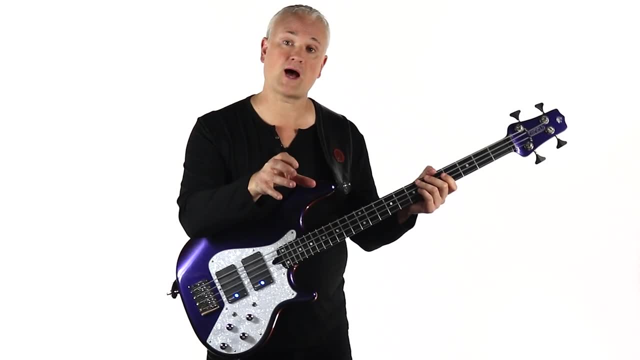 And then we can try two eighth notes: quarter note, half note. So 1 and 2, 3, 4.. 1 and 2, 3, 4.. Then let's try putting the half note at the start of the bar. So half note, quarter note. 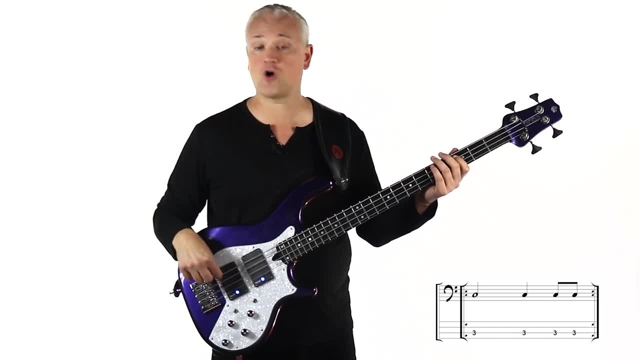 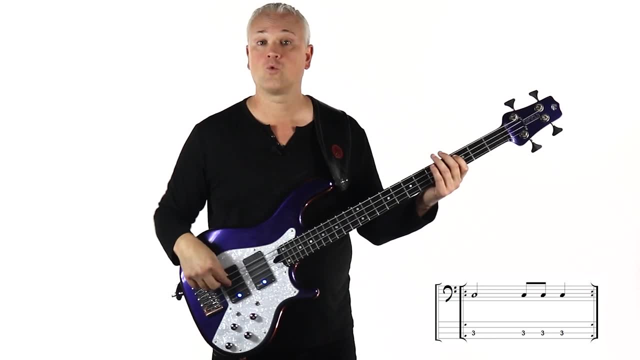 two eighth notes: 1,, 2,, 3, 4 and 1, 2 and 3,, 4 and 1 and 2.. One, two, three, four and And now half note. two eighth notes: quarter note. 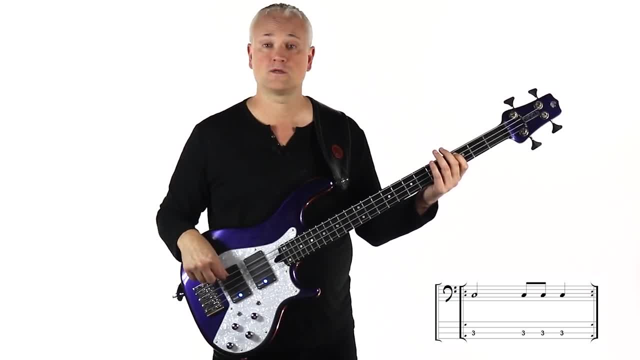 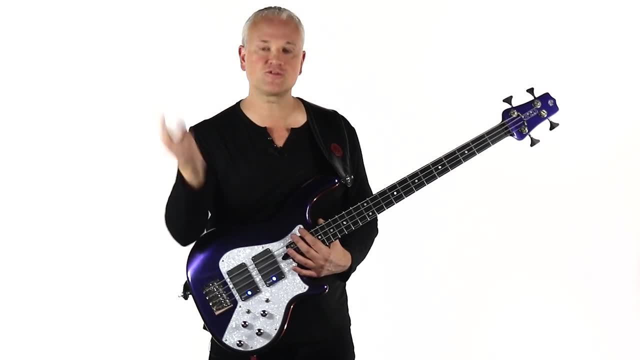 One, two, three and four. One, two, three and four. So remember, those drills are just to aid our counting of the rhythms. So you want to try each of those drills round and round. I know I only played them once through there, but just try them round and round. 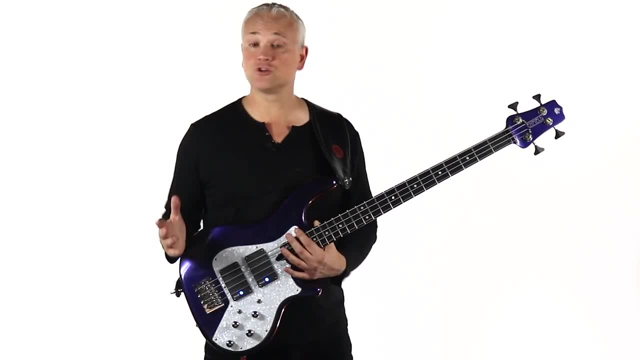 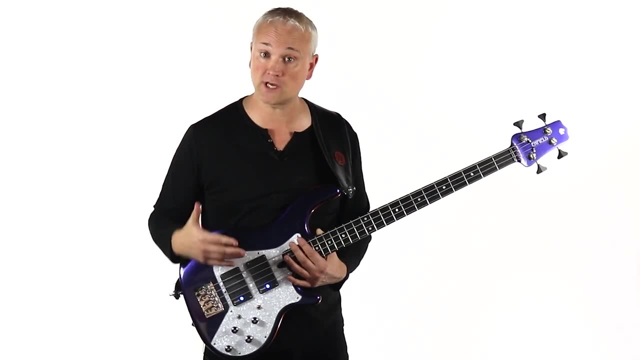 getting used to tapping the foot and counting out the rhythms. As you learn more about rhythms, you'll notice that it's a very organized mathematical system and as you add more and more rhythms into your study, you'll become better at keeping your bearings within a bar. 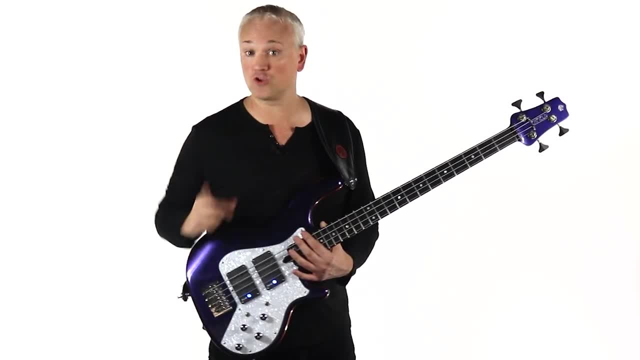 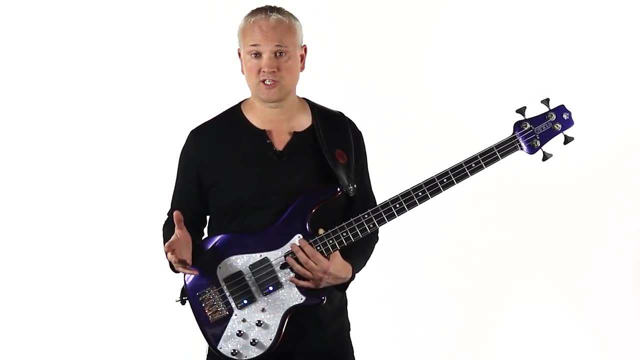 and you'll have a much better rhythmic accuracy and independence. You'll also improve your groove. So that's the basic rhythmic counting up to eighth notes, but there's also the dotted note to consider Now. a dotted note lasts for one and a half times the rhythm specified. 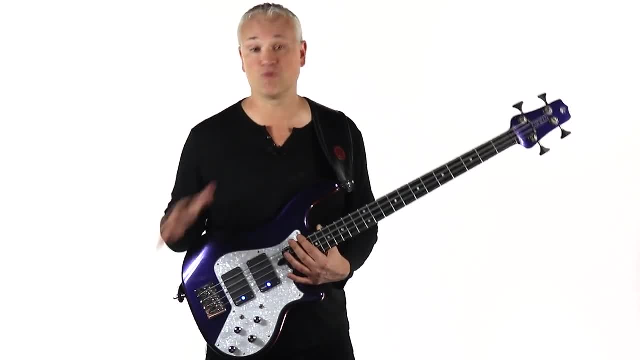 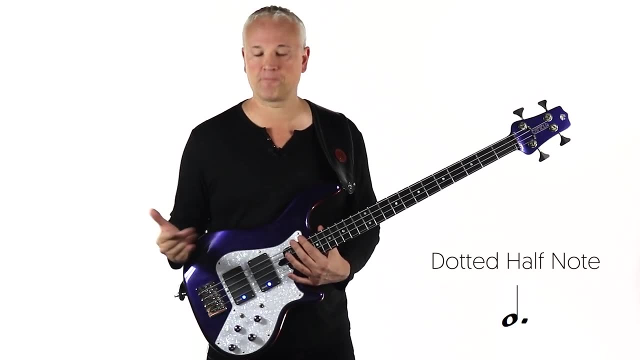 Now, that might sound a bit complicated, but it's actually really, really simple, and you're best just learning to count them in isolation. to be honest, To get started, we'll look at a dotted half note Now. a half note lasts for two beats. 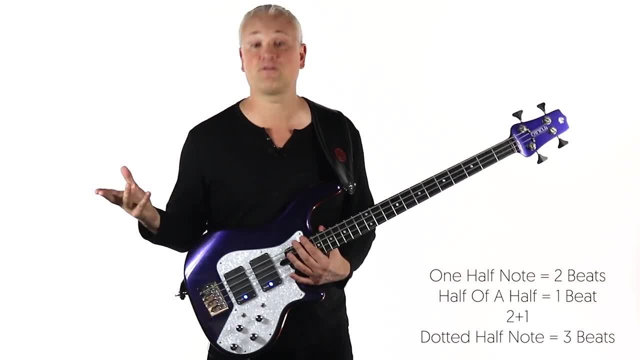 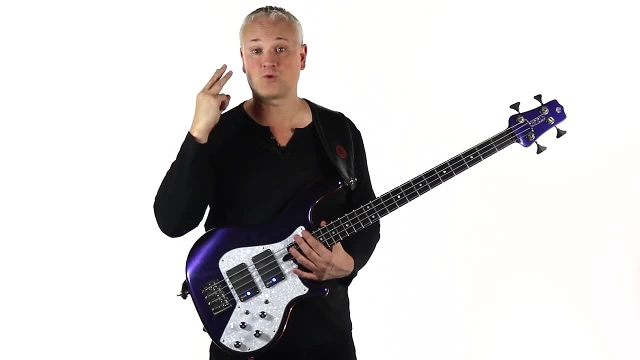 Half of two is one, so we just add that one onto the two to get three. So a dotted half note lasts for three beats and, to be fair, that dotted half note is just there to be able to specify. we want a rhythm with three beats. 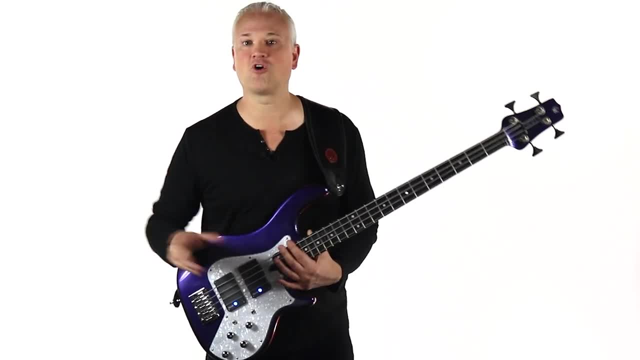 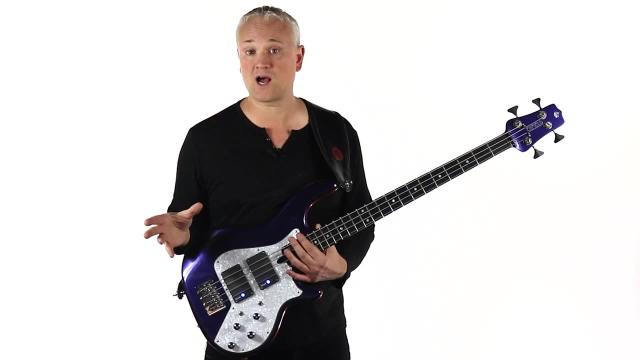 So don't worry too much about the fact that it's half of a half note added on. Really, all you need to know is that it's worth three beats. So in a bar of 4-4, you can only have two rhythms using dotted half notes. 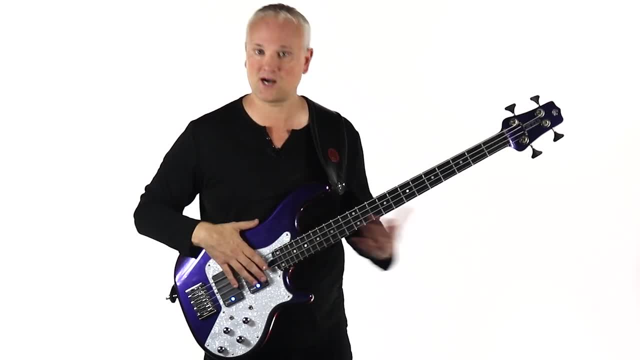 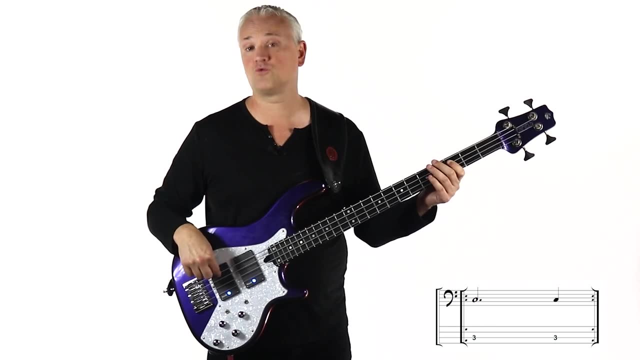 You can have dotted half followed by a quarter, and quarter followed by a half note. So let's try those as rhythmic drills. So first of all, we've got the dotted half and a quarter, so we're going to count that as 1, 2, 3, 4, 1, 2, 3, 4.. 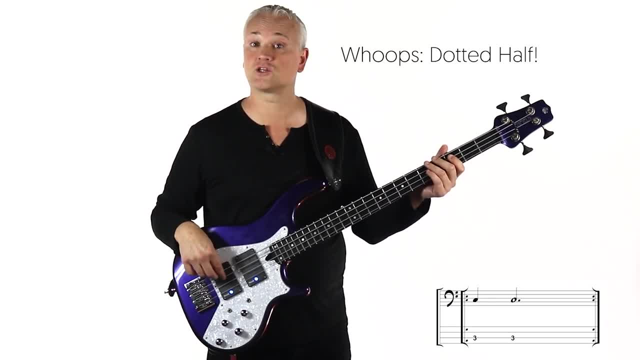 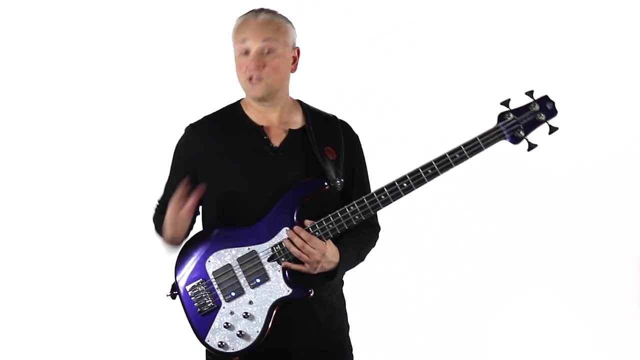 Try that round and round. Then we can try quarter dotted eighth notes. So that's going to be 1,, 2, 3, 4, 1,, 2,, 3, 4, round and round. Next we can try the dotted quarter notes, and this is worth three eighth notes. 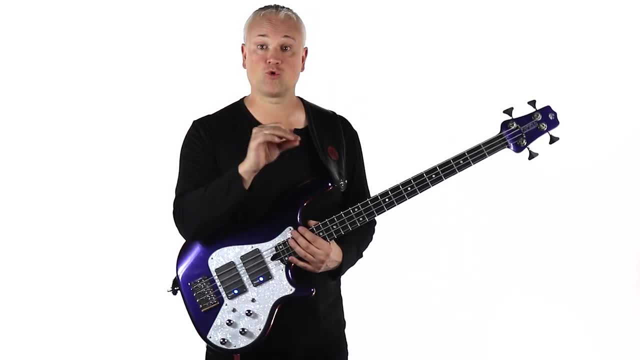 So that gives us two rhythmic cells to consider. We can have a dotted quarter note and an eighth note, and an eighth note and a dotted quarter note. So when we count those for the dotted quarter eighth note, we're going to have 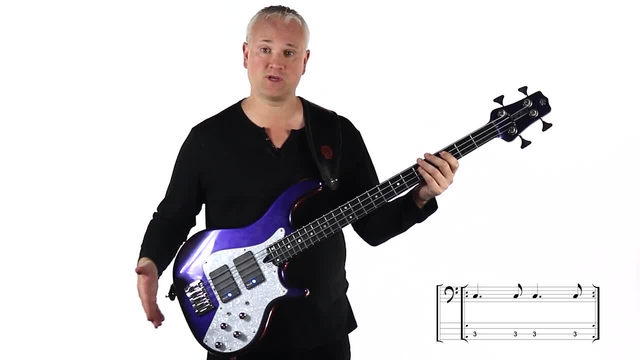 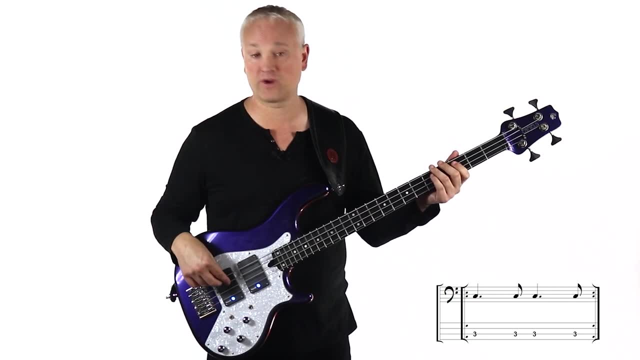 1,, 2, and. Okay, So just count on each beat with the foot and you've got 1,, 2, and So we hit on the 1 and then on the and. And if we were starting on beat 3,, obviously it'd be 3,, 4, and.